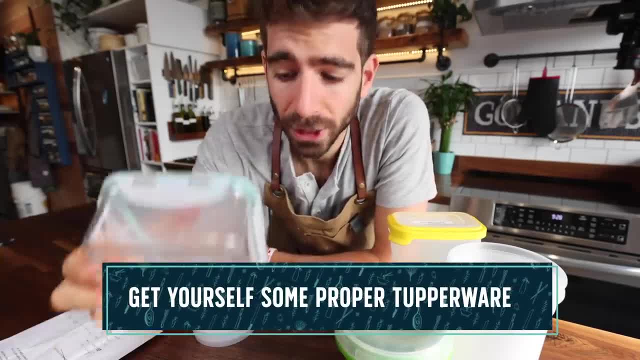 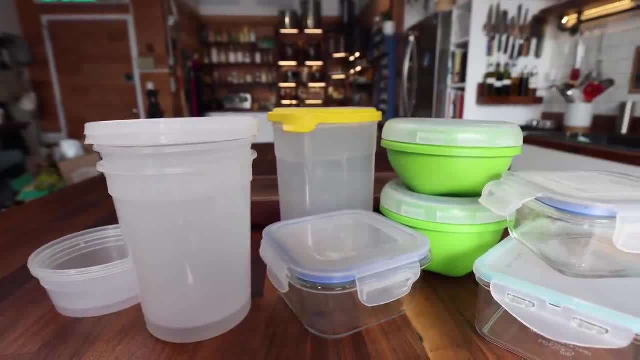 buy yourself some good Tupperware. It is a great investment, Something that's going to keep your food safe locked in and also that will last you many, many years. You're also going to want to get different sized Tupperwares. Having an assortment of sizes is going to make your life. 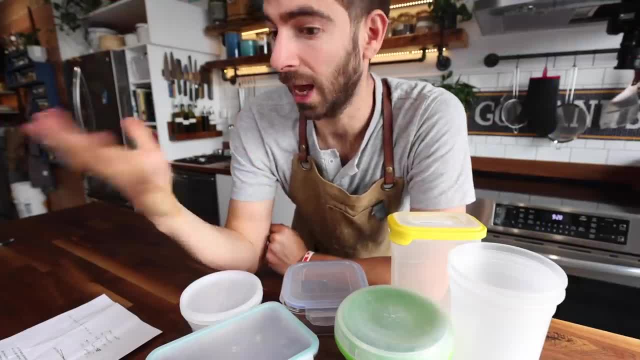 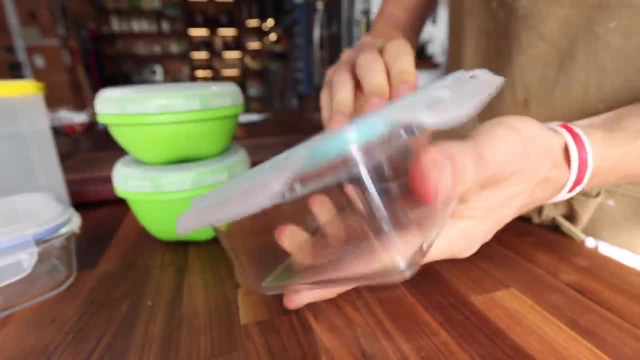 a lot easier. So when you are cooking a certain size of food, well, it can go directly in that one Tupperware and you don't have to put it in multiple Tupperwares. And it's definitely nice to have Tupperware with a strong locking mechanism, because your food will. 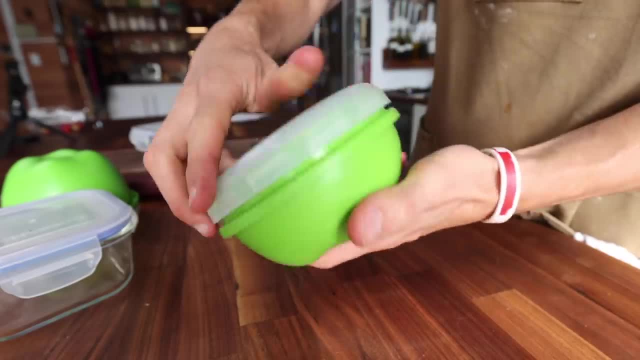 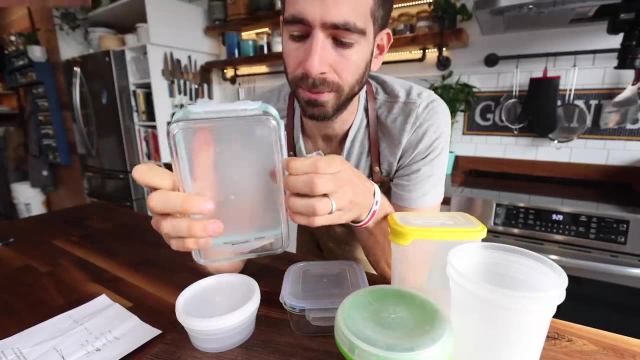 leak, especially if you're traveling with your food. I've had so many cases where I put one of these Tupperwares in my book bag and it leaks, So having that strong locking system is a huge bonus. Get yourself some of these takeout containers in different sizes, but make sure they are. 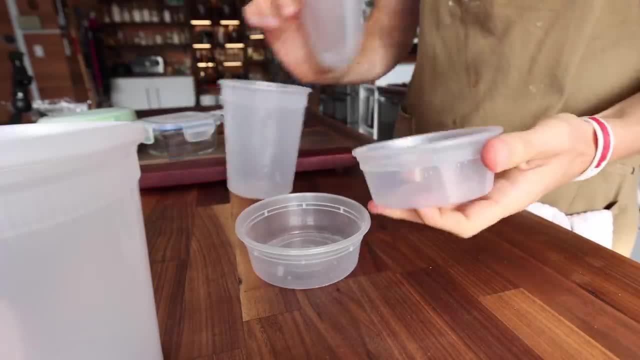 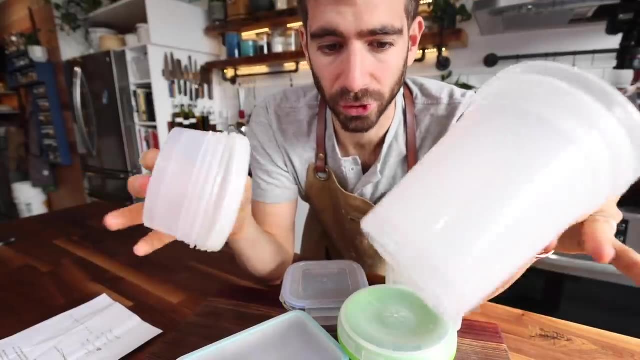 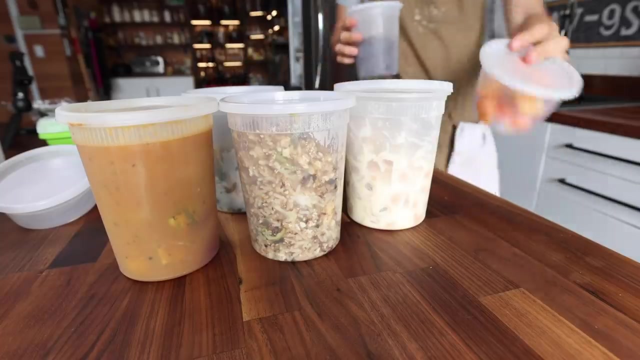 BPA free. These are going to be wonderful for food organization. Having a ton of these that I can reuse has completely changed my kitchen and fridge organization. because you just want maximum storage. There's always something to put away And if you aren't organized things can get pretty sloppy in your fridge or your pantry. 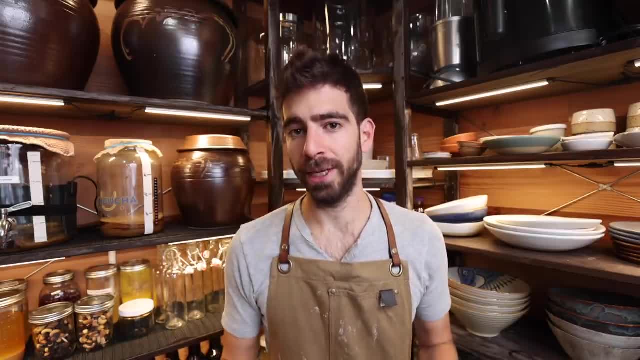 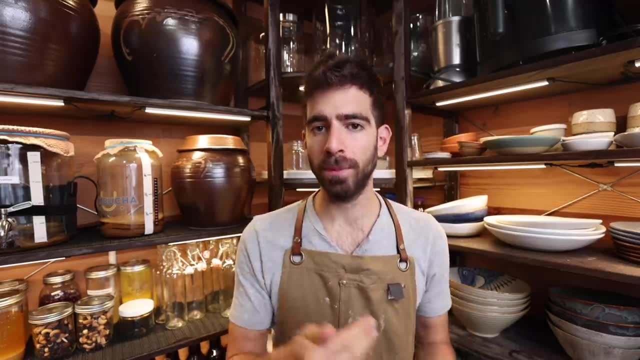 The number one excuse I hear from people for not cooking is being too busy, And we're all busy people. but being busy is not a good excuse to not get in the kitchen, because it's amazing how much you can get done in a very short period of time. 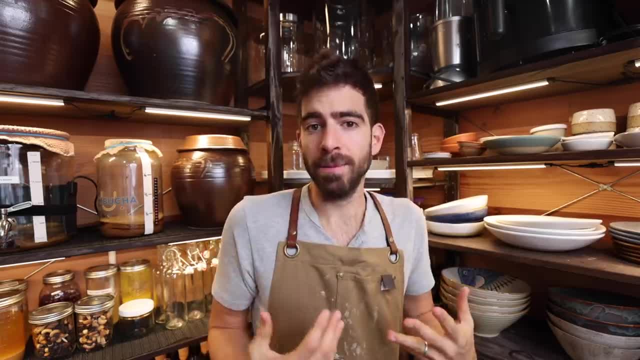 whether it's just a few hours on a Sunday or for me. I have a baby, So when the baby goes to bed it's like I'm in the kitchen. I'm getting you know breakfast, prepared lunch, whatever it is. 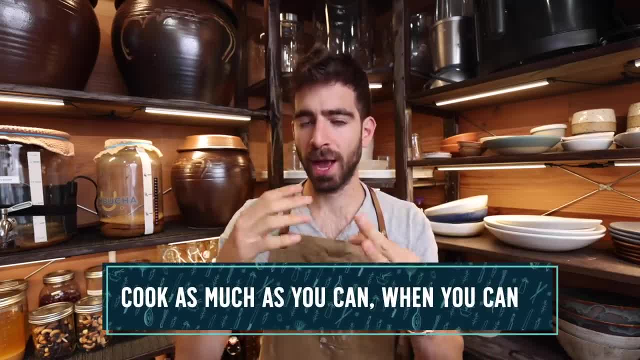 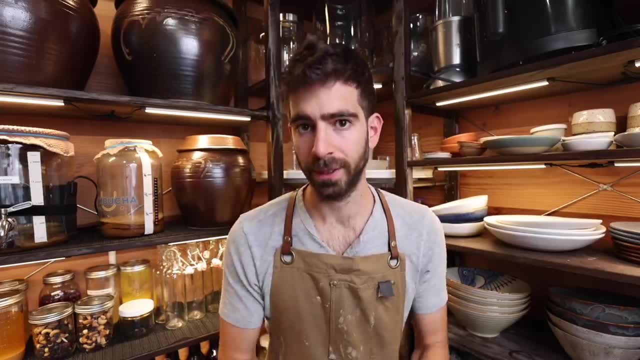 So that's my next tip: Get it done when you have the time. You have to get in that kitchen and just start working And I'm telling you, you will be very surprised how much you can get done in a short period of time. Why am I standing by the spice rack? Well, I'm tired of you eating boring. 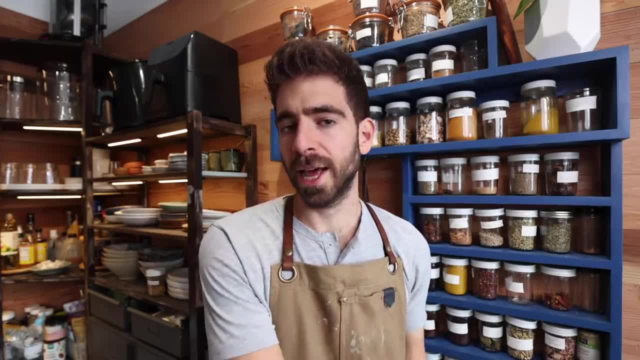 and bland food all week, And one of the easiest ways to fight against that is to make one all-purpose spice mix that will make your food taste better. One of the easiest ways to fight against that is to make one all-purpose spice mix that will make your food taste better. 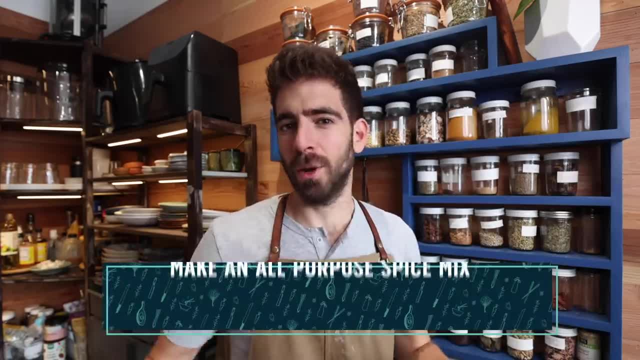 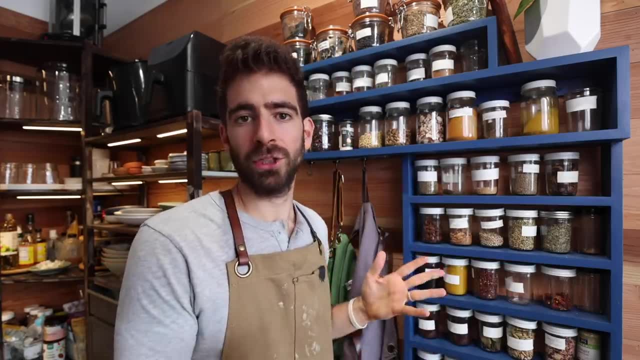 One of the easiest ways to fight against that is to make one all-purpose spice mix that will make your food taste better. It's going to come in handy with so many different dishes and it couldn't be easier to make. All you have to do is pick out a bunch of spices And for me, I just have fun with it. 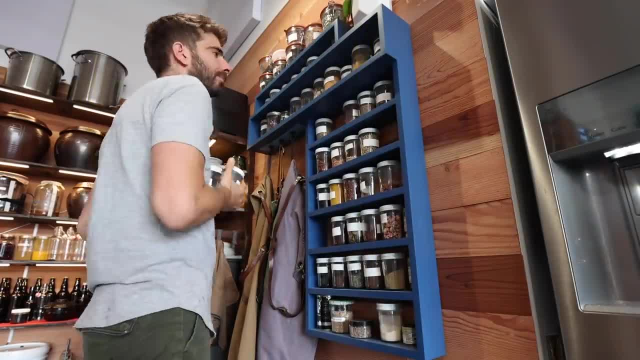 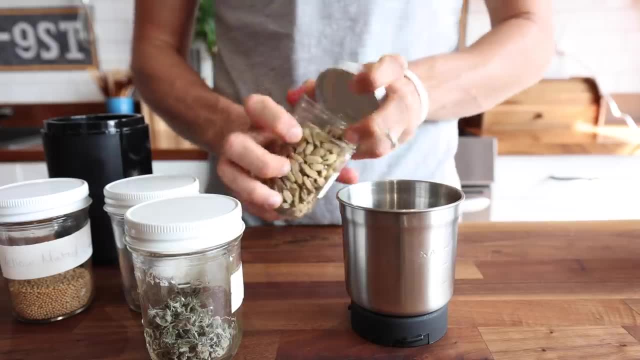 trying different combinations every week. There's really no wrong when it comes to making a homemade spice mix. I'm going to use a spice grinder, which I recommend every pro home cook should have, but you can use a mortar or pestle, or you could just use pre-ground. 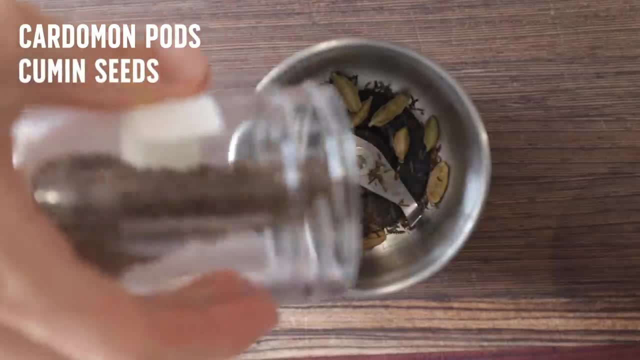 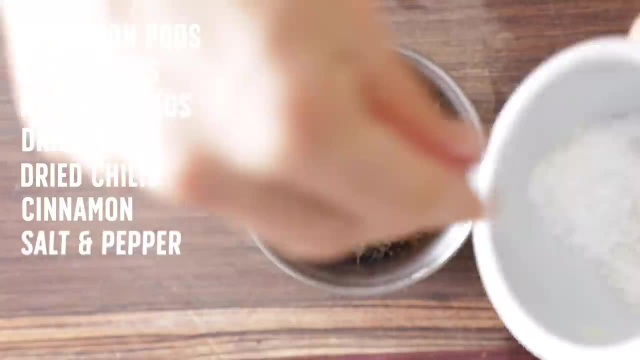 spices and mix those together. I'm adding some cardamom pods, some cumin seeds, some mustard, some mustard seeds, some dried thyme, dried oregano, dried chilies, a little bit of cinnamon and salt and pepper and grind that up until I had a nice consistency And you'll see this spice mix. 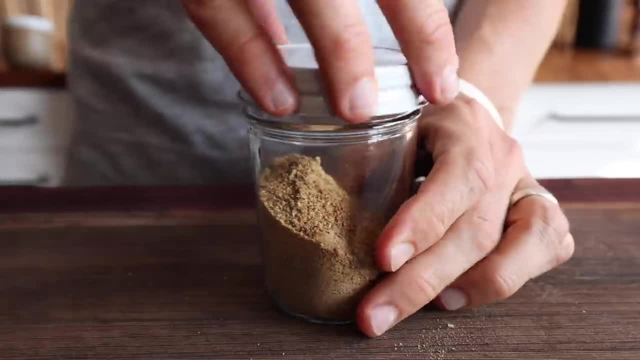 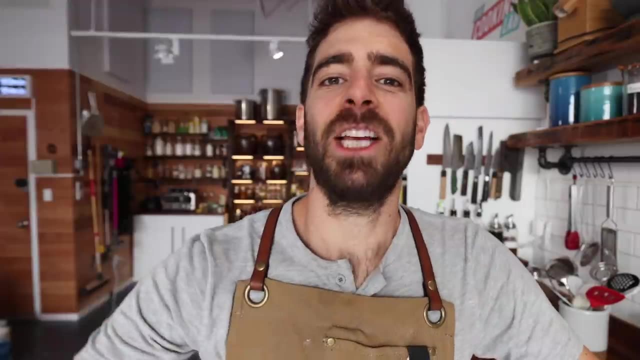 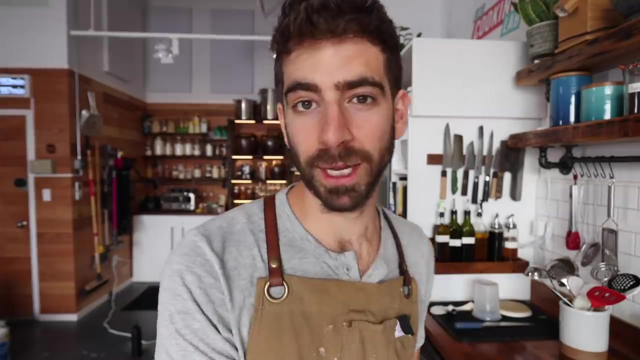 come up throughout this video. I'm always a bit confused when people comment in and they tell me cooking is too expensive, which is ridiculous. The amount of money I've saved being in quarantine over the last few months, being forced to go to work and being forced to go to work, and being forced to go to work. 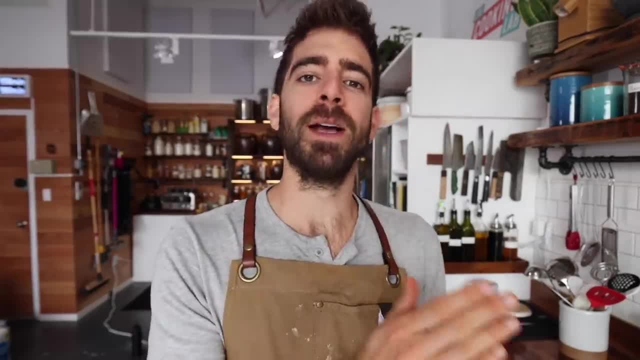 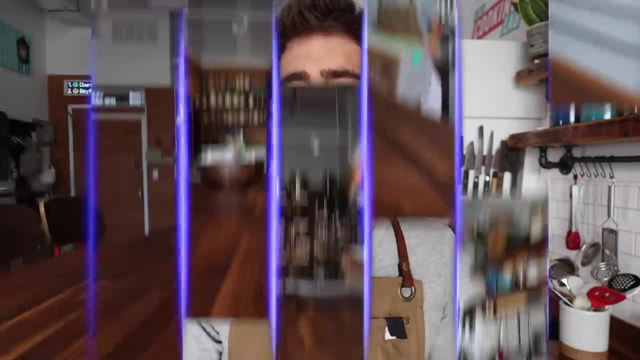 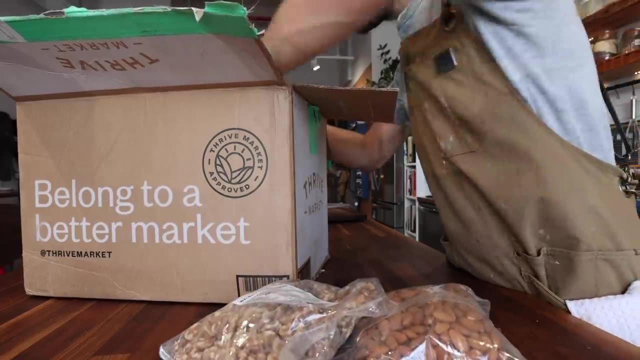 best ways to do. that is the sponsor of today's video, which is Thrive Market. Thrive Market is an online membership-based market on a mission to make healthy living easy and affordable for everyone, And I'm a big fan of Thrive Market because it's just an enjoyable online shopping. 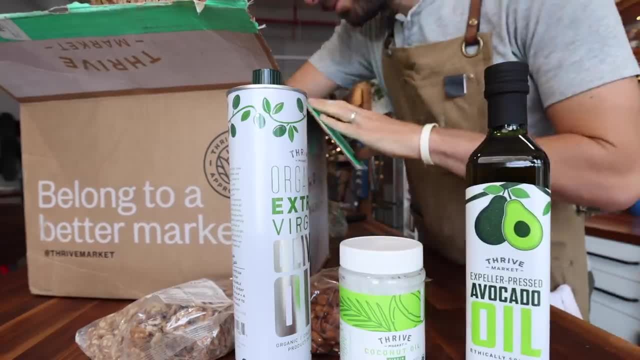 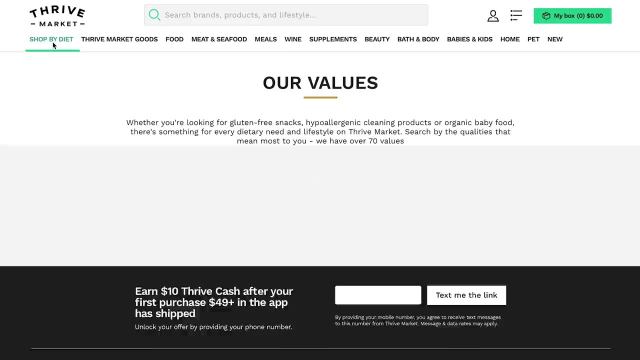 experience. I know I can count on them for having quality products, organic products, healthy snacks, whatever it is, And you can actually break up your shopping experience to fit your own personal needs, whether it's a paleo diet or keto or vegan or BPA-free, Whatever it is. 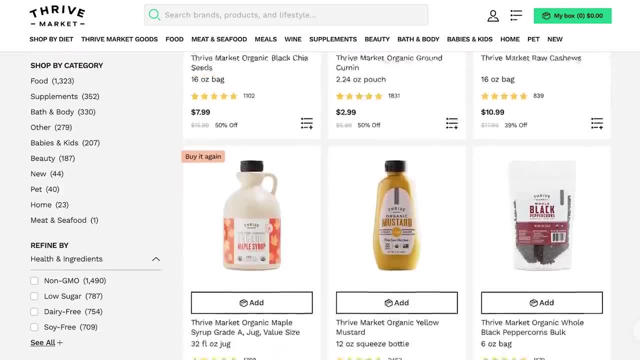 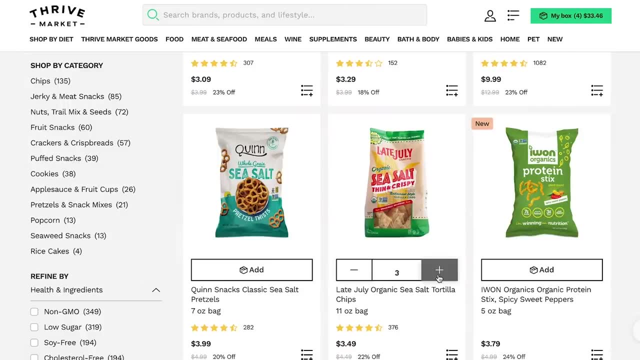 it's really easy to search And they have such an incredible variety of products, which is great when you're building out your pantry and you don't have to go anywhere, which is a huge bonus. I love a well-optimized food shopping experience that you can just pick out your stuff and boom. 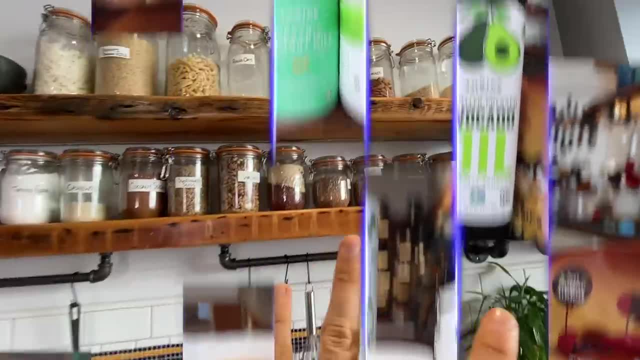 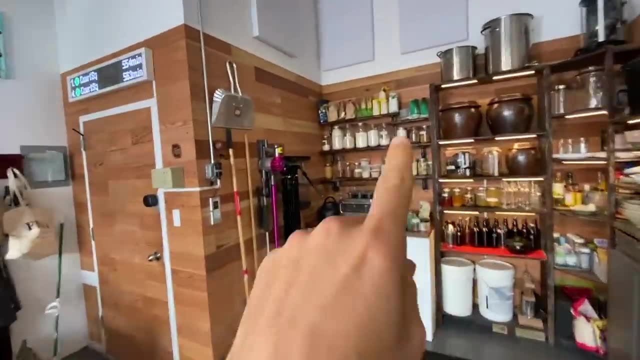 it shows up and you can Stock out your pantry. This is what I'm talking about: The stock pantry. This is options, These are savings over here, All potential meals. Even if we come over here, we've got a whole bunch of. 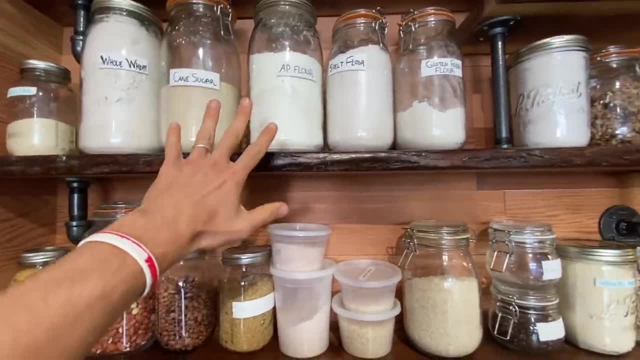 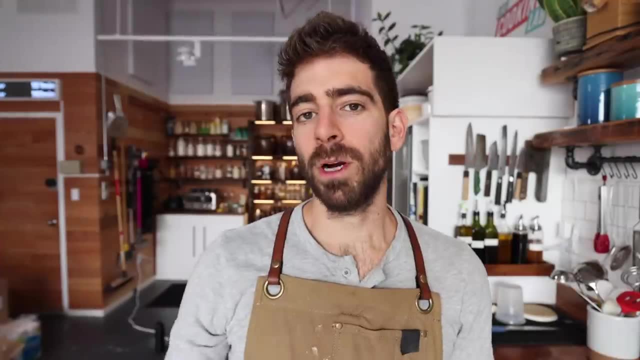 different grains we can use in dishes. We have different flours for baking, We've got popcorn- all types of stuff, So many options for pantry items, And Thrive Market offers different types of memberships to fit your own personal needs. So you can choose a 12-month membership or you can just do a one-month membership For me. I went with the 12-month, which came in at $5 a month, And if you click the link below in the description and join Thrive Market, you'll get a free gift from Thrive up to $24 in value. 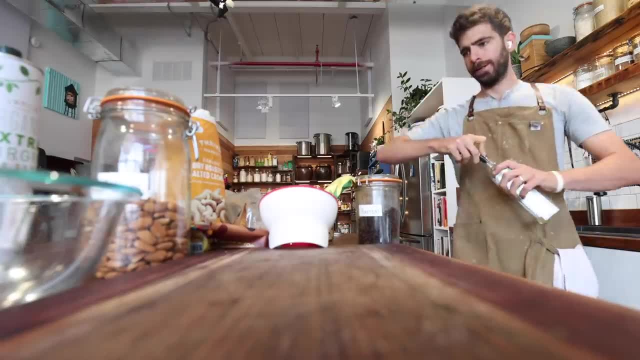 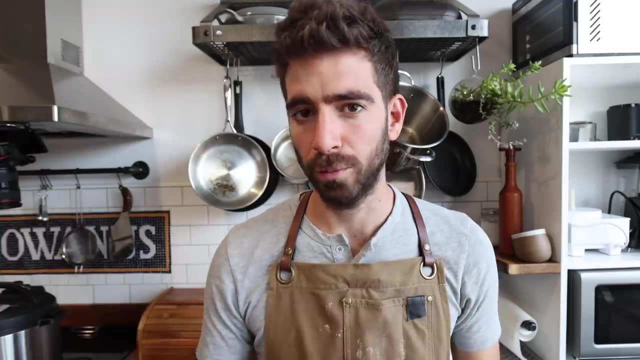 So, now that my pantry is stocked, I've got my Thrive products. Well, it's time to go. It's time to start meal prepping and start saving over time. One of the biggest mistakes I see when it comes to food prep is people just running out of food, which then leads to the problems of ordering. 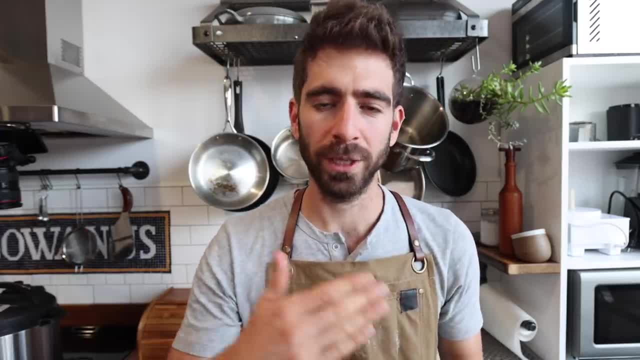 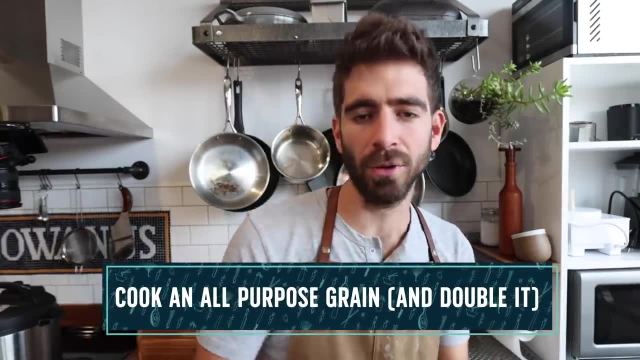 out spending a ton of money, which we're trying to avoid, And one of the best ways to do that is to have a base grain in your fridge, cooked and ready to go and have a lot of it, Something like a rice or a lentil or a quinoa. Think of it as like a really good pair of jeans Once you have. 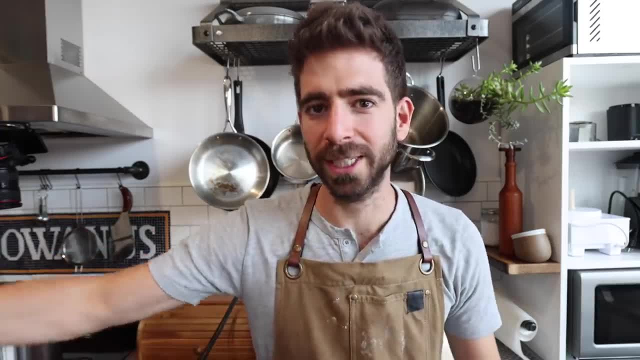 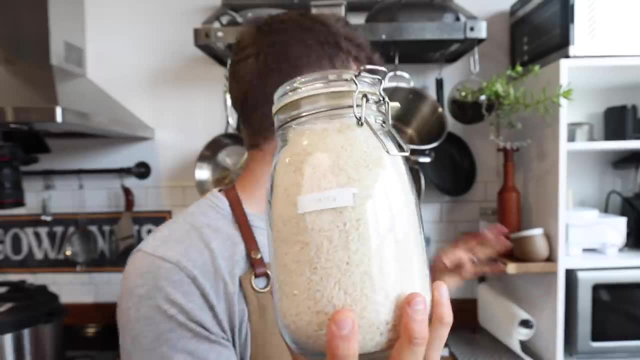 that pair of jeans. well, you can just throw on a shirt or throw on some accessories and build off of it, but you need that base. I'm going to be making some standard long grain rice. There's so many uses for this And all I need is a pot for some perfect, fluffy rice. So the first step. 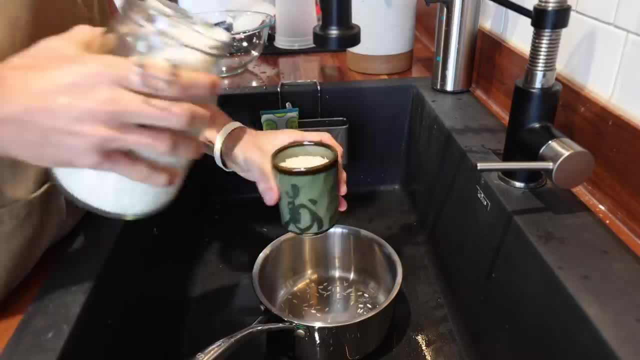 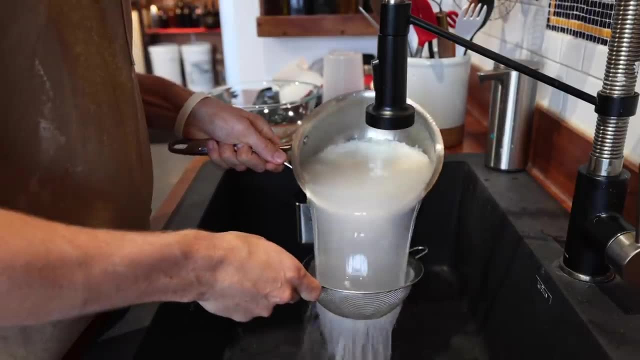 is to take some type of cup to measure out your rice- Again, I'm doubling this- and pour that rice into your pan and make sure you wash your rice. There's a lot of starch on rice And if you want gloopy rice, well then, skip this step. But if you want perfectly fluffy rice, make sure you wash it. 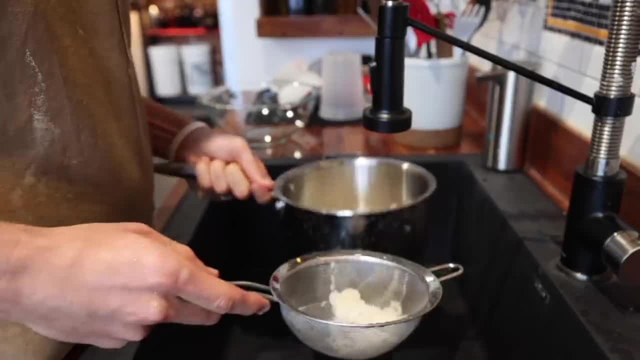 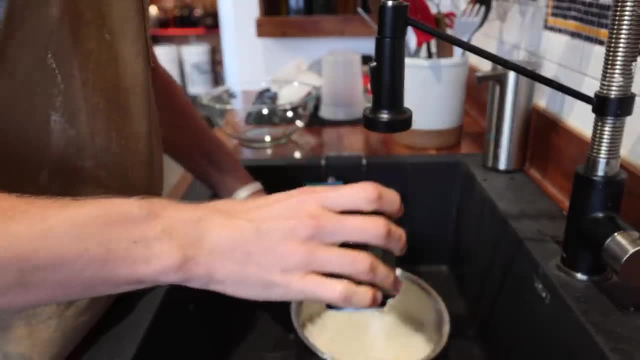 until it runs clear. Once your rice is washed and drained, you can put it back in the pot, And I'm going to take that same measuring instrument and double the amount of water, minus a little bit, because there is still a lot of water left over from washing the rice. 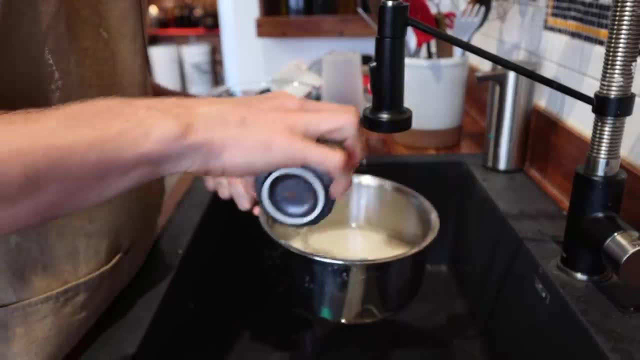 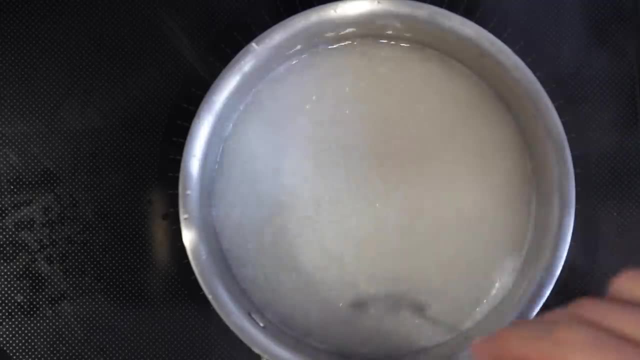 So if it's one cup of rice, you're using just under two cups of water. Bring that up to a boil, stirring it just a few times so it doesn't stick to the bottom, And then, when it hits that boil, you can put a lid on it and turn your heat down to the lowest it goes and let it cook for 15 minutes. 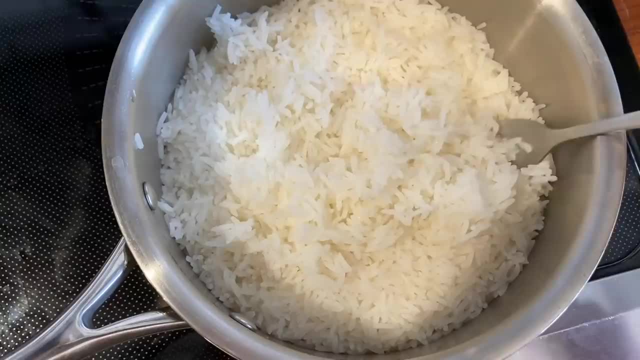 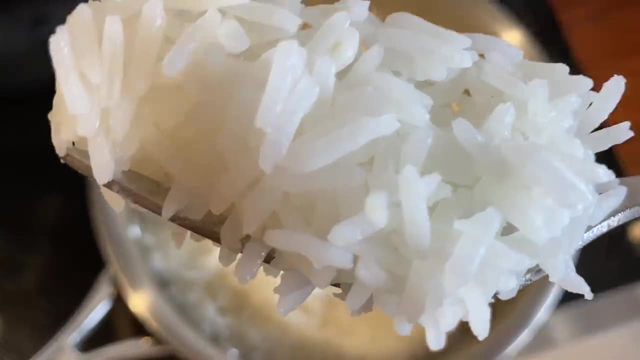 and then turn the heat off And you can let that rice steam in there and just continue to cook off the heat for another five minutes And there you go: Perfect, fluffy white rice, ready to turn into so many different dishes. Speaker 1. 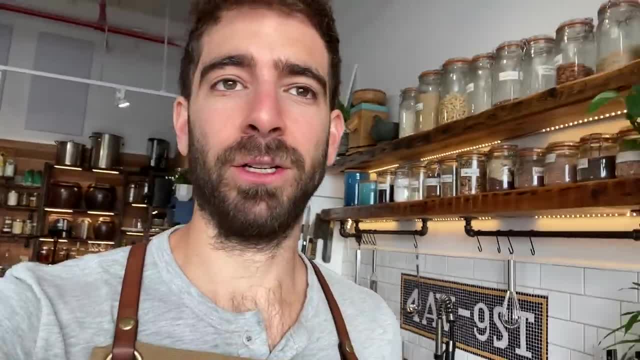 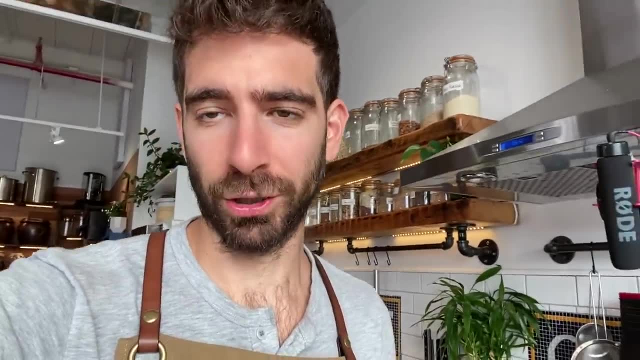 I feel like when people start cooking for themselves, they're almost shocked at first how much food they actually need, And they end up burning through all of their food very quickly in like one or two days. So you need to cook a lot of food, And one of the best ways to do that is 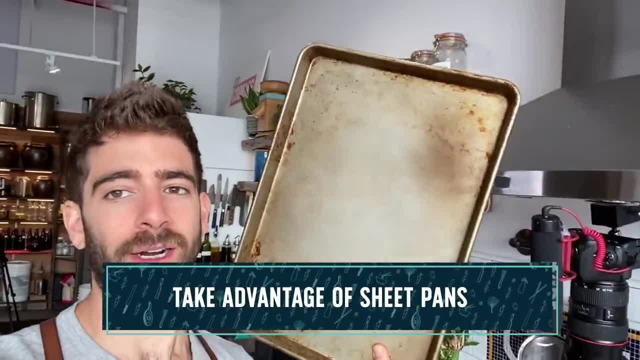 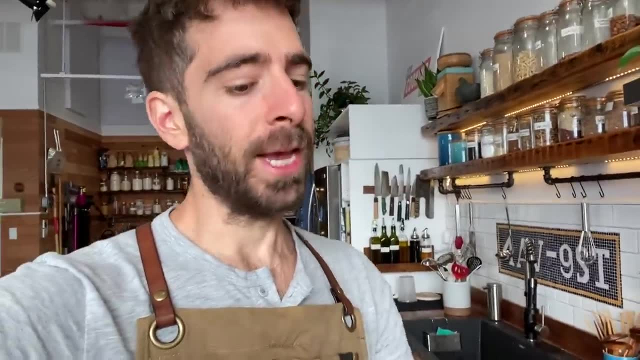 to take advantage of sheet pans like this, because look at all that surface area. we throw a bunch of veggies on that in the oven. boom, we've got a lot of food. And that's exactly what I'm going to do, for my meal prep is roast some veggies, And the best part is you can do everything on. 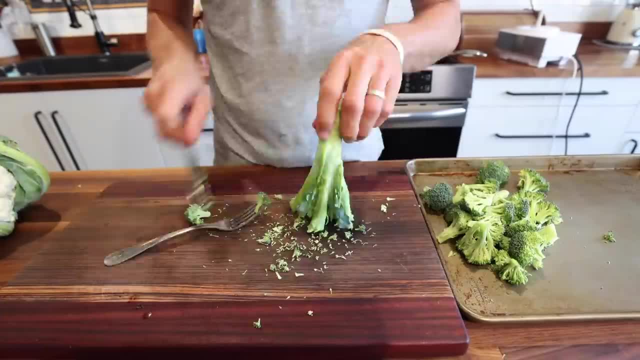 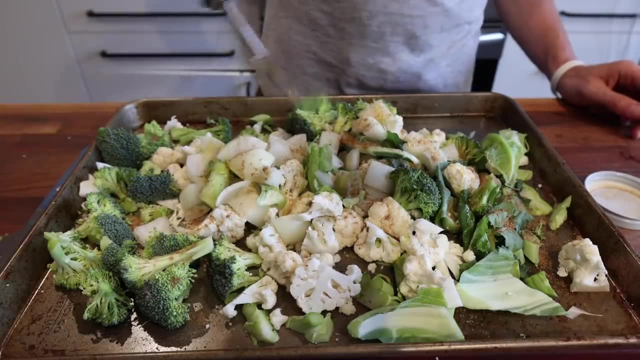 this sheet pan. So I've got some broccoli. chop that up, including the stems. they're delicious roasted. cut up some cauliflower and some onion, added that to my pot, hit it with some oil and a great place for that flavor blast spice mix to really enhance these veggies. mix everything up. 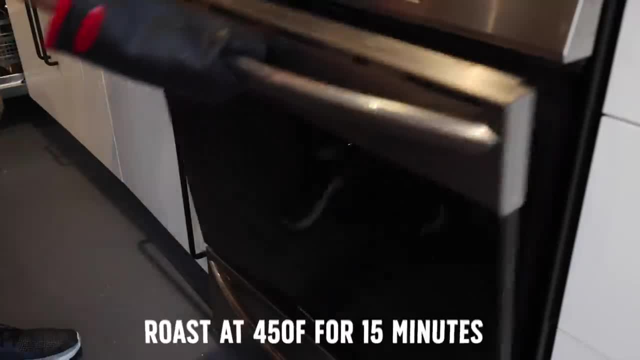 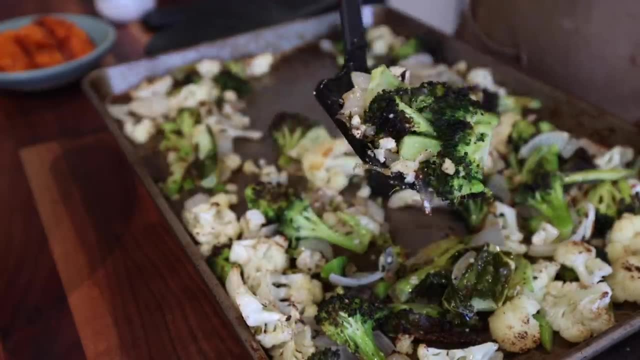 right on the sheet pan until it was well coated and threw that into a 450 degree oven for about 15 minutes until I perfectly roasted veggies. then you can just toss those in a Tupperware and use them in different dishes. Speaker 2. 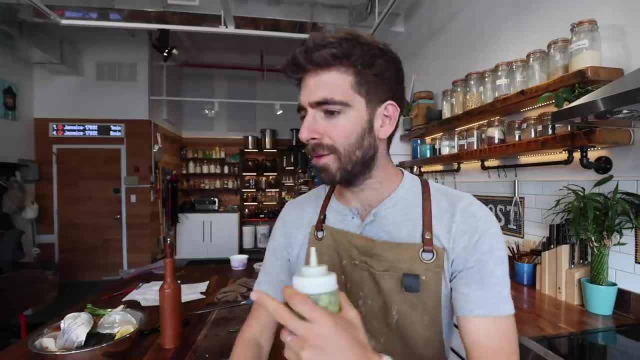 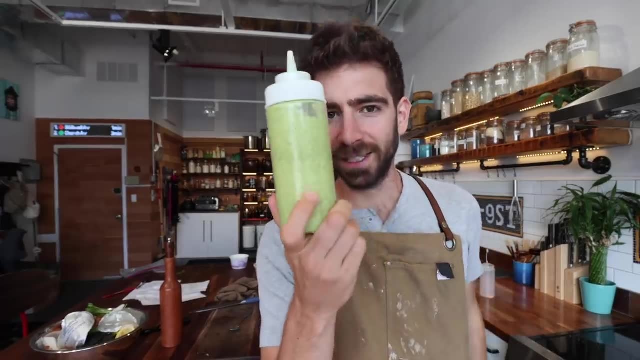 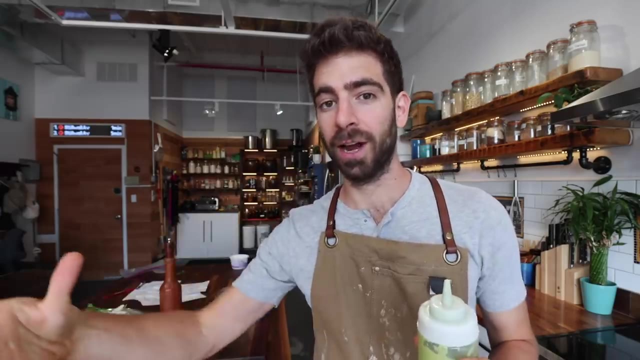 is all week long. Like I said, with that spice mix, it is all about finding simple ways and hacks to just make your food taste better, And one of the best ways to do that is an all purpose sauce. you make one sauce that you can pretty much put on anything throughout your entire week. So 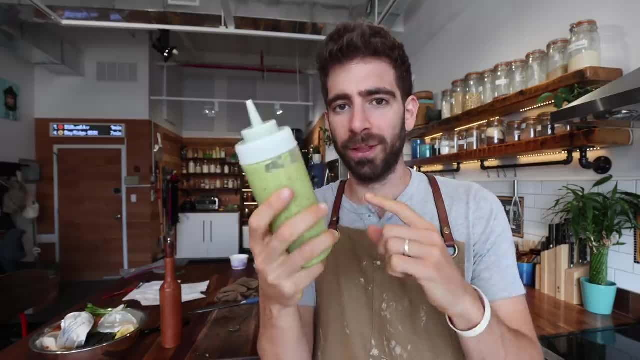 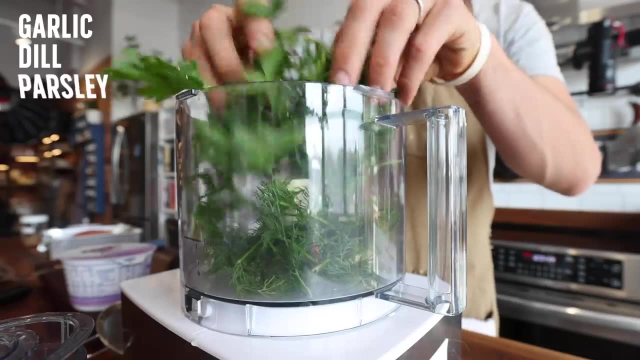 I'm going to teach you this recipe, which I love. it's pretty much a healthy rant. you replace the yogurt with avocado. So to make it is really simple, I'm going to take out a food processor, add one clove of. 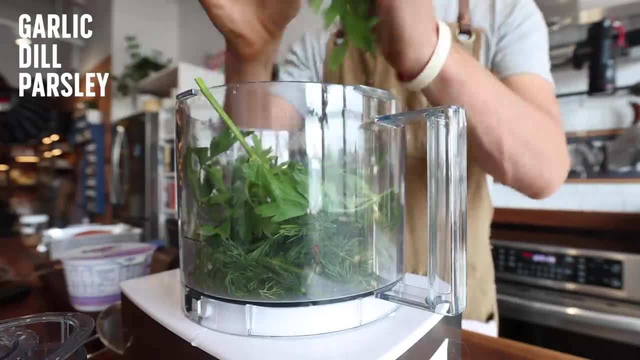 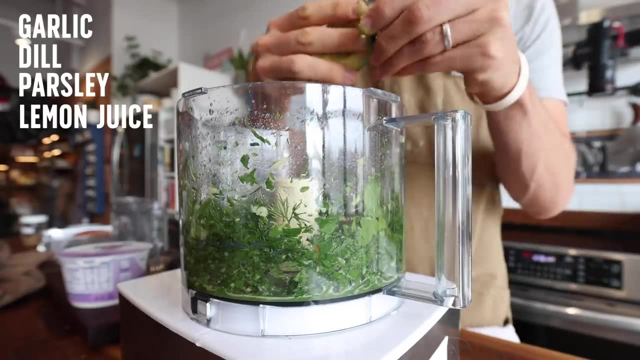 garlic and a bunch of dill and parsley. The herbs are key to really give it that flavor. I squeeze in the juice of one whole lemon and started processing that until it broke down a bit. Then I added in one avocado, which is a great way to replace Mayo and make it a little healthier. 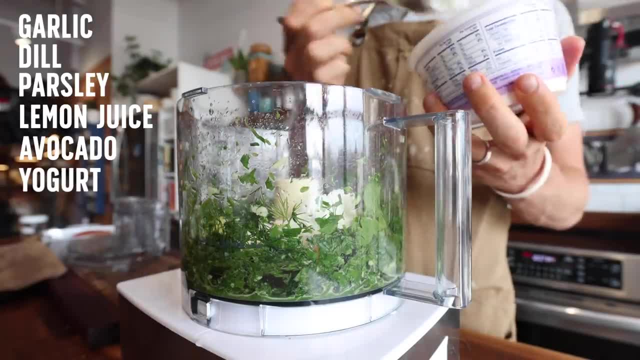 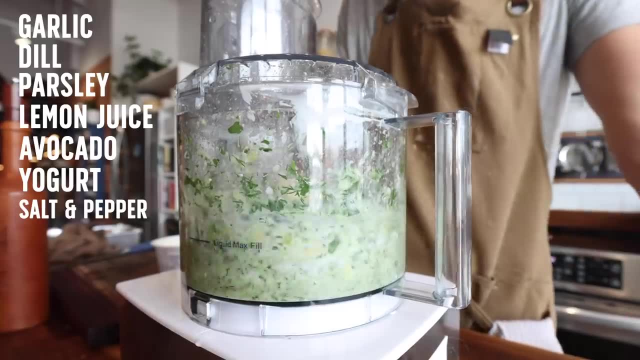 but you still get the fattiness and the creaminess. And then finally, a few spoonfuls of yogurt and salt and pepper, And I blended that until it came together and checked out the consistency, And at this point I can adjust the consistency with. 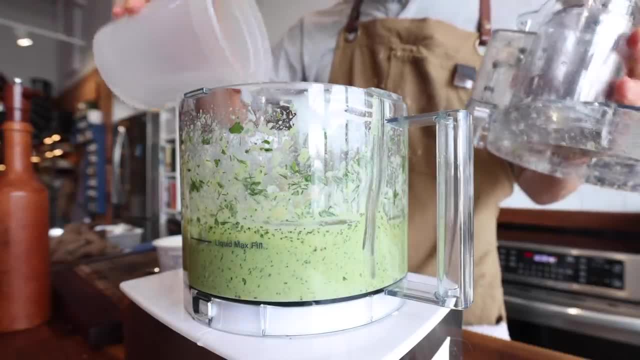 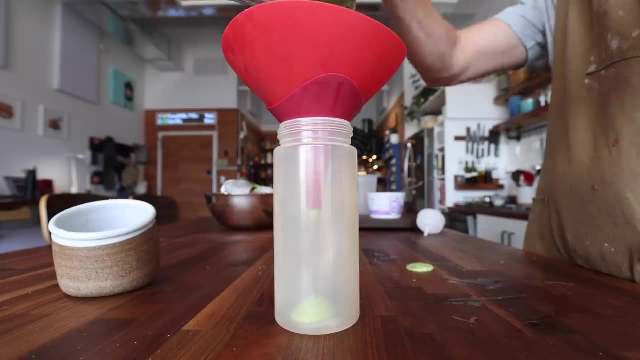 either more citrus or more water, which I used in this case, until I get the perfect consistency that I'm looking for. I'm milking this funnel because this sauce is a little thick And if you want to turn this into a salad dressing, just add a little more citrus or 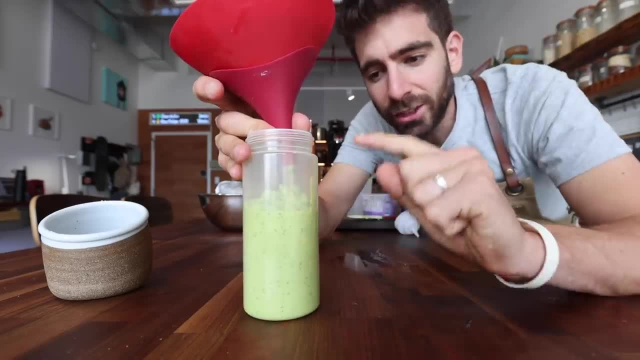 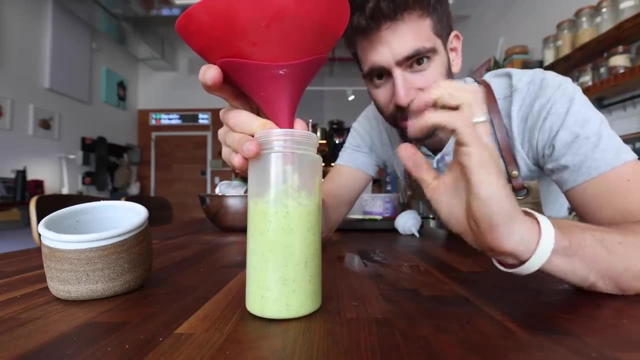 just add more water. But I love this type of all purpose sauce because I could sauce up some seared chicken, throw it on top of some veggies. And that's what I'm going for when I make one of these all purpose sauces, thinking about something that can have multiple uses throughout the week. 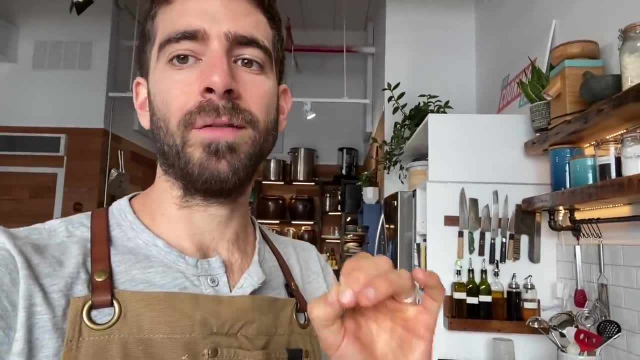 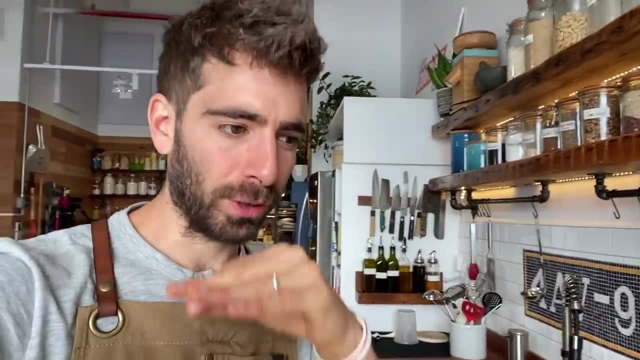 And speaking of cooking a lot of food, one thing I really like taking advantage of in the kitchen for meal prep are machines like this: pressure cookers, slow cookers, anything that's going to make your life easier, something that you can set it and forget it so you can go work on other meal. 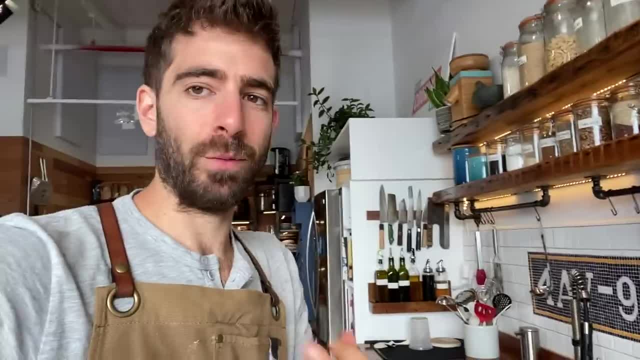 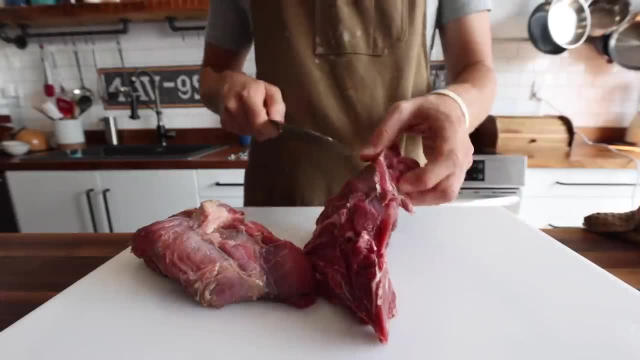 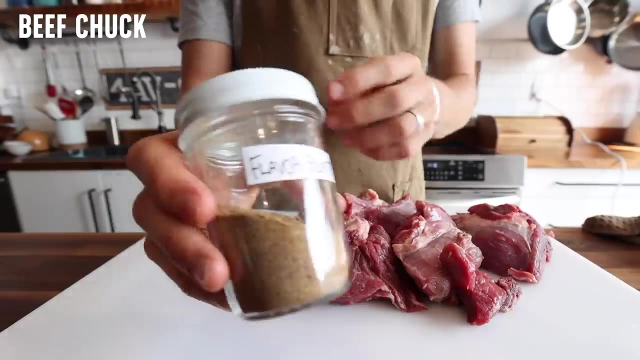 prep. So what I'm going to do is slow cook some meat, because if we have a bunch of slow cooked meat, well that is just great food, great protein to have throughout the week. So I've got some beef- cooking type of cut will work great for this- And I coated it again with the flavor blast spice mix. 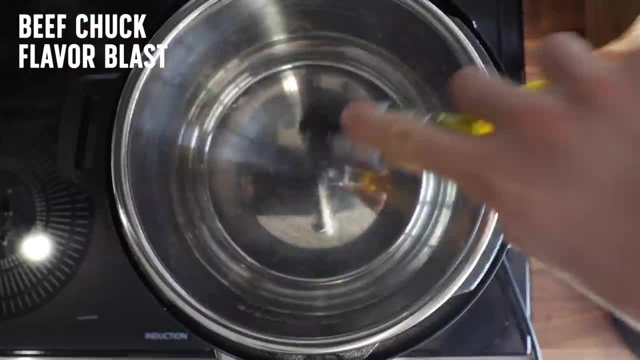 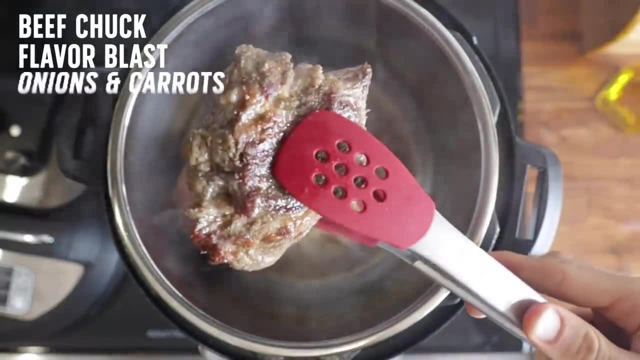 coming in handy with multiple things already. Then I seared that off inside my pressure cooker to build a little extra flavor, which I would highly recommend, And then threw a bunch of ingredients in there. I've got some onions and some carrots, some garlic and just a little bit. 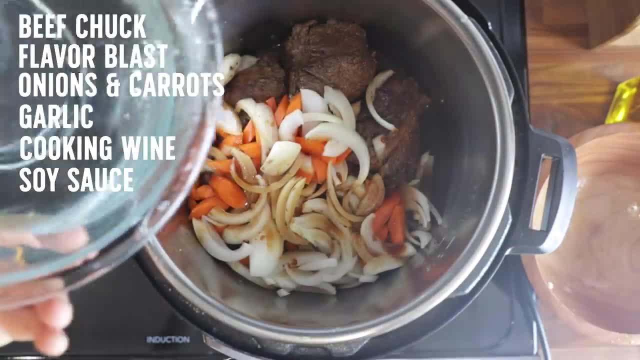 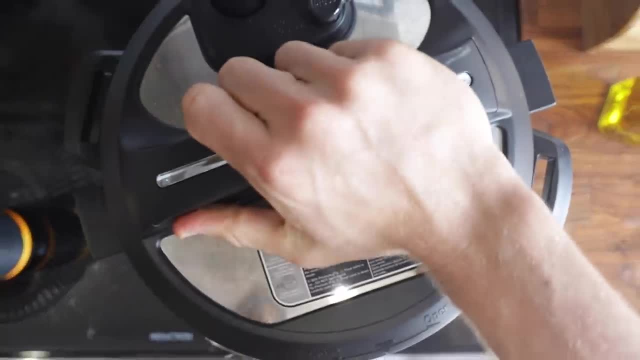 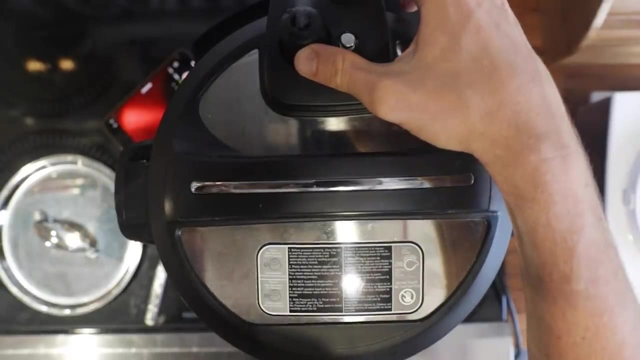 of cooking wine and some soy sauce. I'm keeping it pretty simple here. I'm not making a stew, I just want the meat. So I put that on pressure cook for about two hours. And of course you can slow cook that over hours and still forget about it. But for me I've got a bit of a time crunch, so I'm 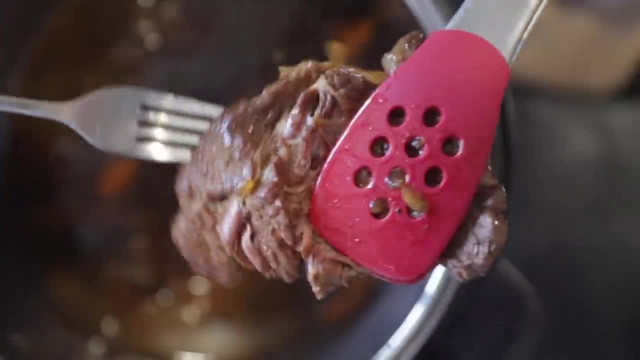 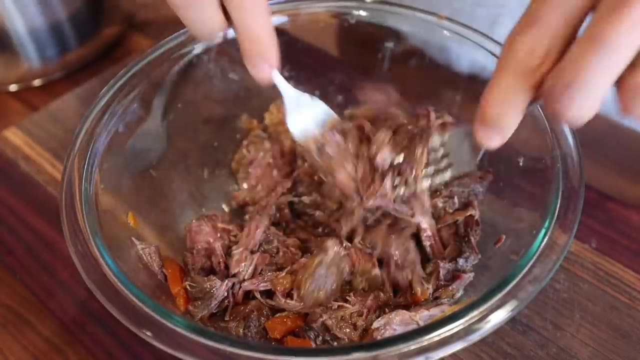 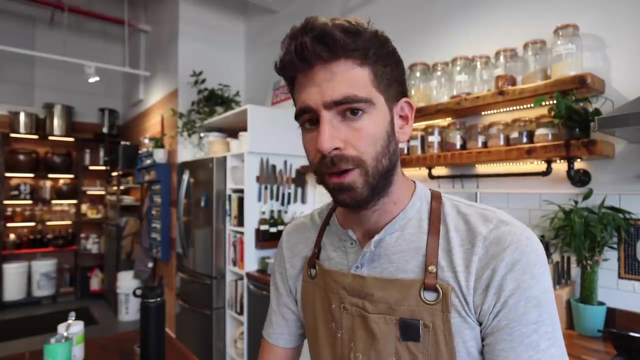 going to pressure cook And after two hours I have beautiful tender beef that is going to provide some really good sustaining meals over the week. So the next few tips are all trying to accomplish the same goal, which is giving you some ideas on how to eat healthier. 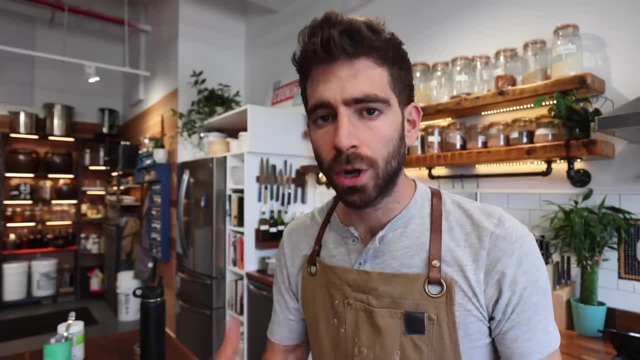 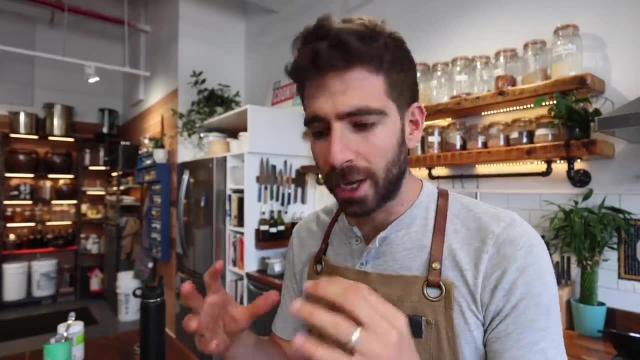 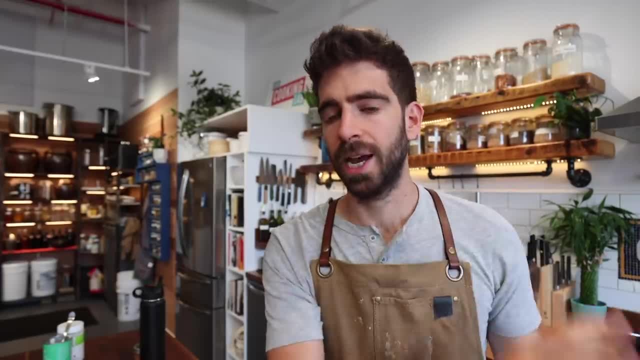 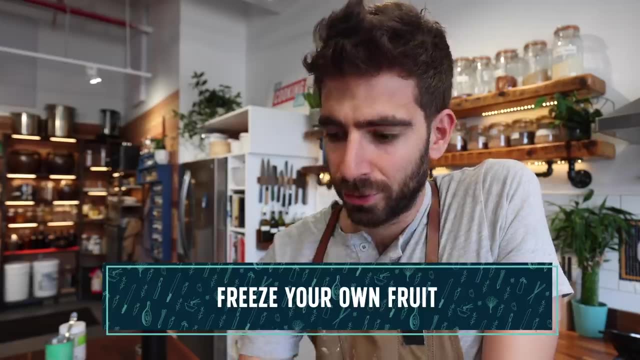 good, healthy food is going to give us the energy to perform those tasks much better. So the first thing I do all the time is I freeze my own fruit, which is great because once you have that frozen fruit, you can just eat it and snack on it. You can turn it into smoothies or 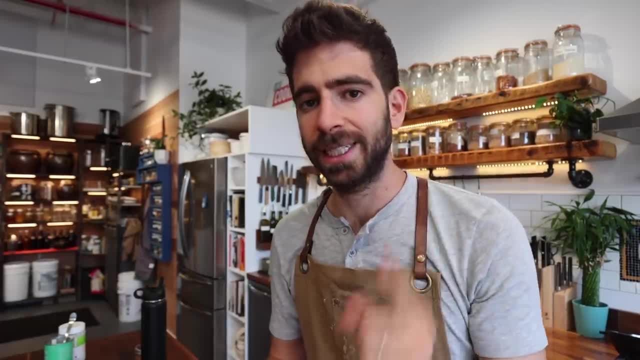 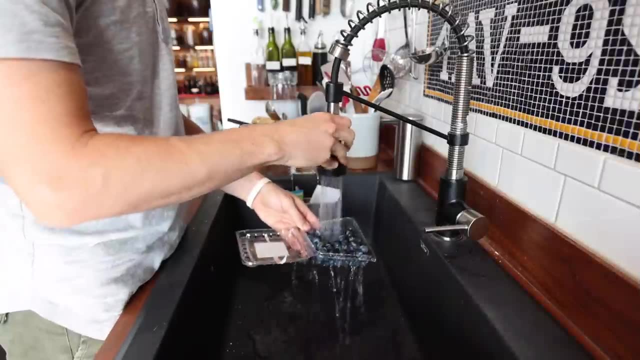 you can make healthy snacks out of the fruit, which you'll see in a second. But rather than just getting fresh fruit and throwing it into a bag, you're going to want to follow this tip, which is taking your fruit, washing it off, making sure it's dry before it goes in the freezer. 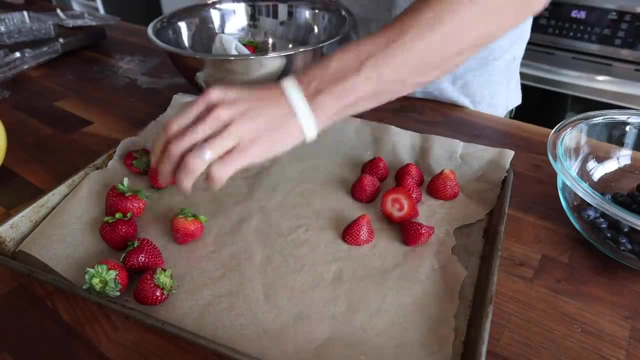 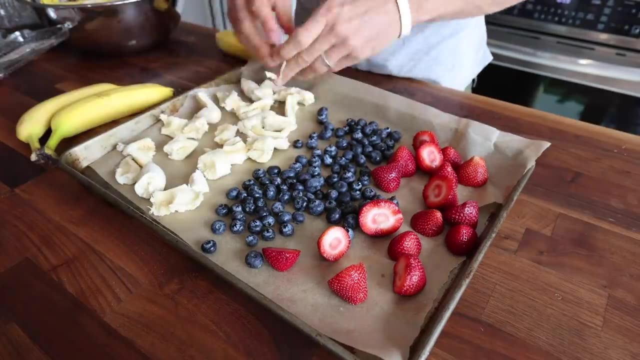 and then put it flat on a sheet tray, And what this is going to do is it's going to freeze each piece individually, So when you then put it in a container or bag, it's not going to clump together, making it much easier to use straight out of the freezer. 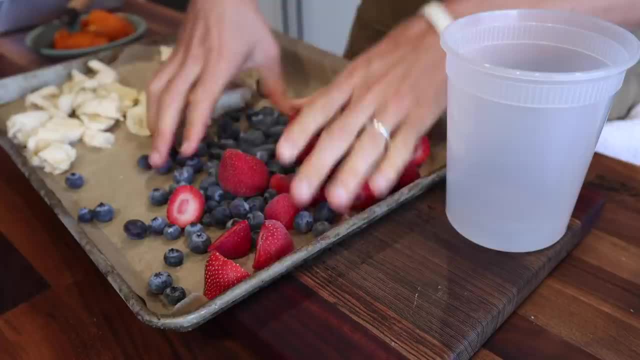 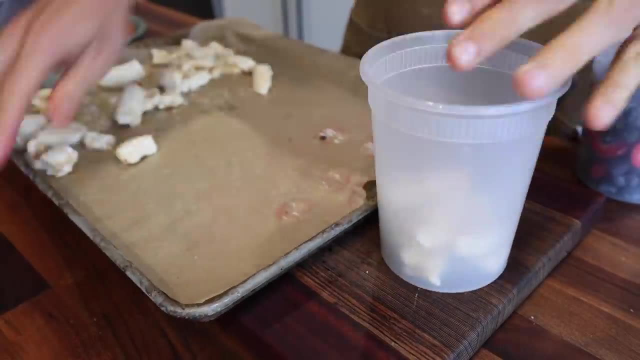 Now, of course, you can make a fresh smoothie for breakfast or just a nice little energy kick, But also it's just extending the shelf life, and frozen fruit, just as is, is a really good snack if you're feeling a little hungry. And speaking of snacks, that is my next tip. 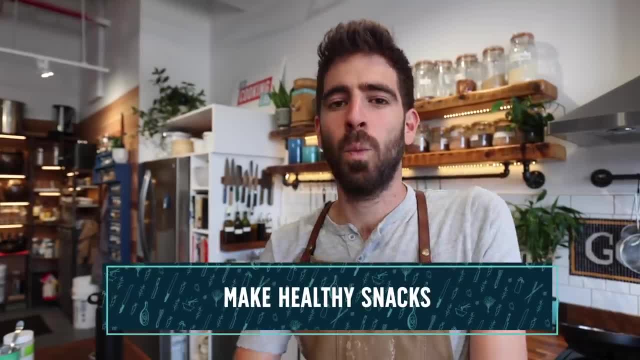 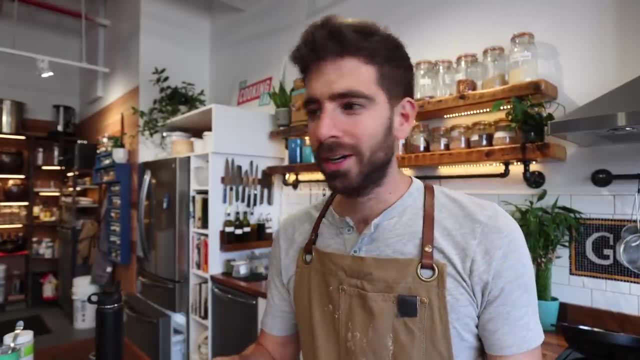 You got to have healthy snacks around. This is one massive mistake that I see with so many people: If they don't have healthy snacks in between meals, that's when you're going to get a little naughty. You're going to get into the cookies, the chips, whatever it is, and you can go downhill. 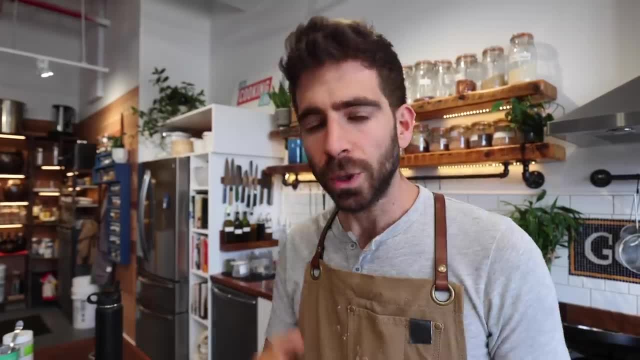 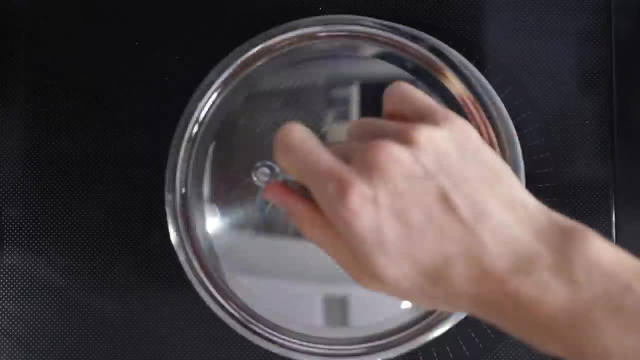 and crash in the middle of your day when you're trying to work. So here are a few of my favorites that I make all the time. Number one is just popcorn. I pop my own popcorn and boom. what are we going to use? That all-purpose Flavor Blast spice mix is such a great. 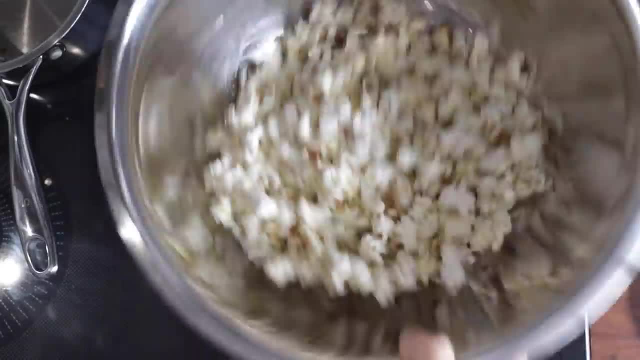 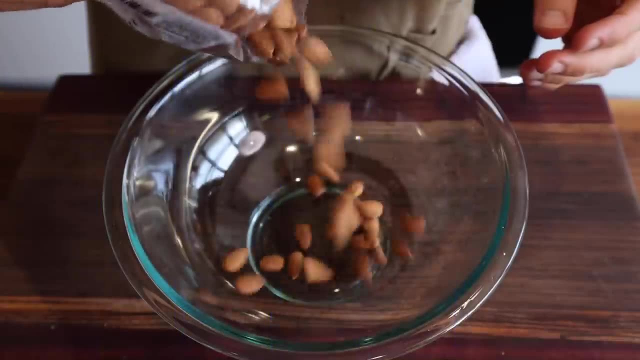 way to take this popcorn from something that's all right- just salted popcorn- to an incredible munchie. The second snack is so simple that it's almost ridiculous, but I would get so jealous when my brother would whip out a batch of homemade trail mix. He always traveled with homemade trail mix. 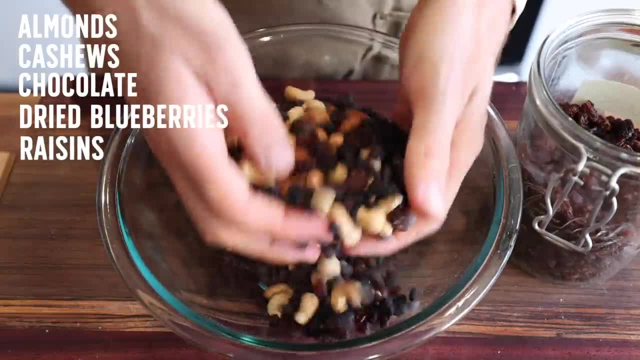 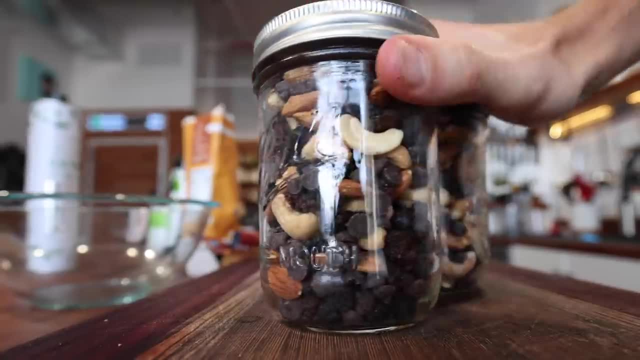 and it's just a great thing to have around when you need that little salty or sweet kick. but you can control all of the ingredients going into it and you can customize it in whatever way you want. Now my third healthy snack might be my favorite of all time: the ultimate guilt-free. 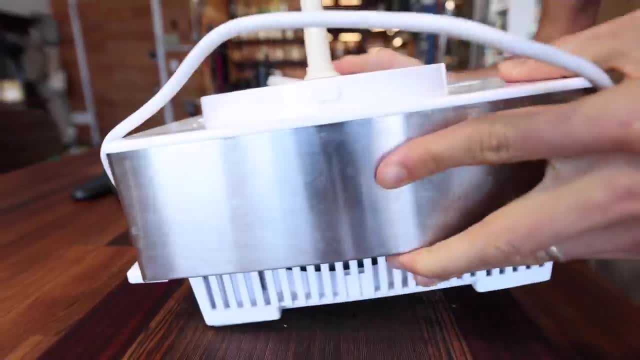 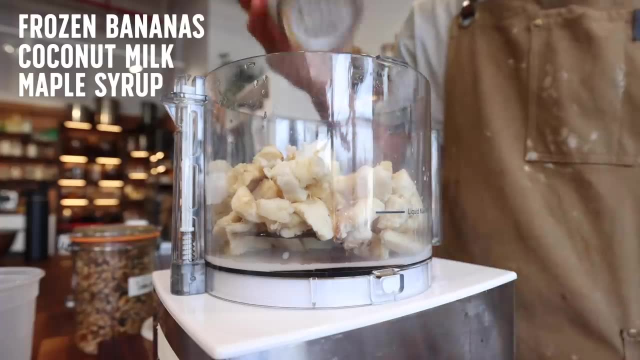 ice cream, and we're going to be using those bananas that we just froze. Throw them in a food processor along with some coconut milk and some maple syrup, and then I hit it with a little bit of salt- because I like my ice cream salty- and give that a blend until it is silky. 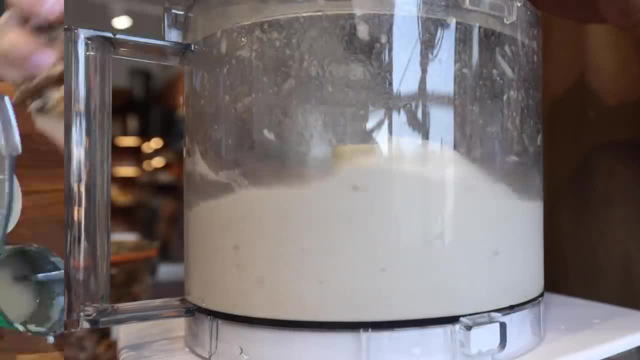 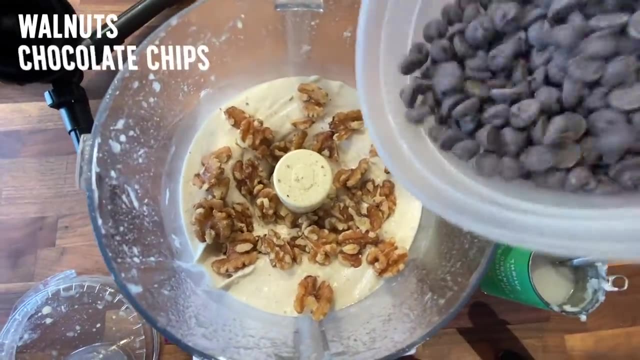 Now I prefer texture in my ice cream, and a great way to get some texture in this is just add some nuts. I'm going to add walnuts because they go great with bananas, and then chocolate. I can't resist chocolate, and these chocolate chips are sweetened with stevia, which is also a great. 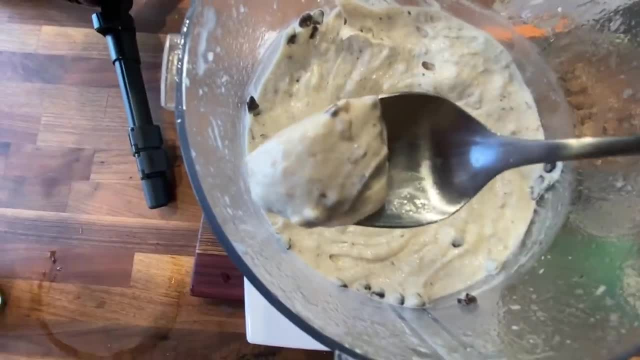 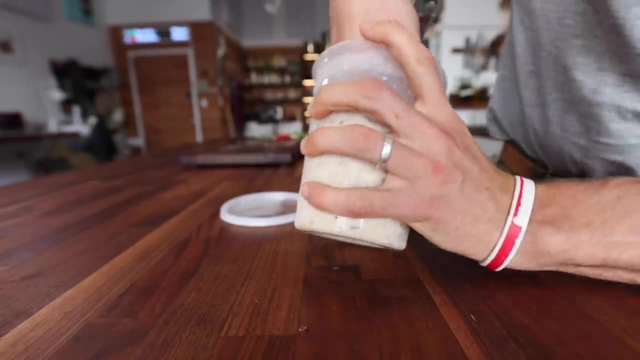 little hack and then I just blend that up until those ingredients are roughly chopped, and I transfer that to some type of Tupperware and put that in the freezer until it's hardened, and then you're ready to serve that up all week for an incredible. 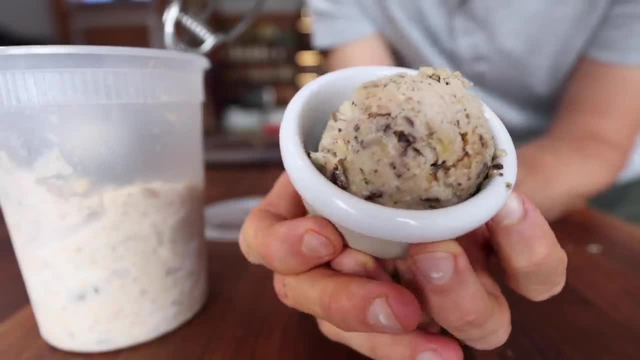 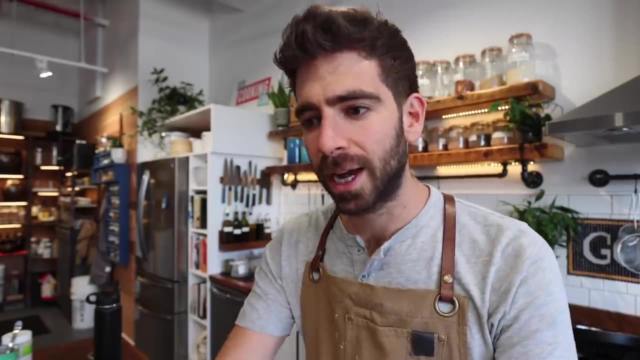 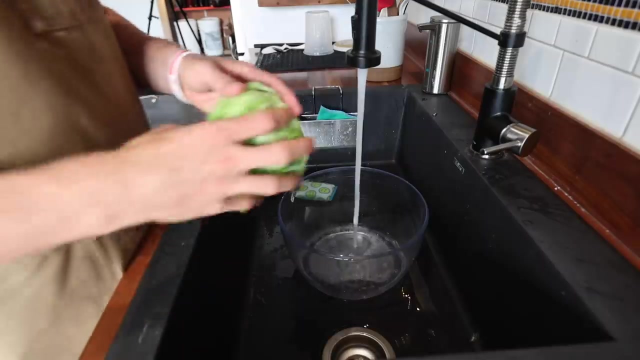 guilt-free ice cream. So the goal of meal prep is to really nail down a balance of foods, and I find if I'm lacking some raw food in my diet I just don't feel as good. I just need some raw veggies in there. so what I like to do is, in the beginning of the week I'll buy one or two. 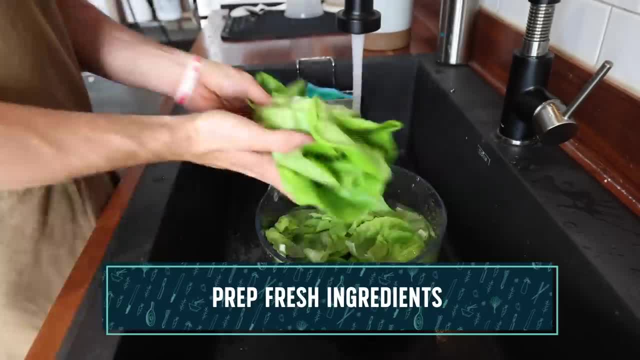 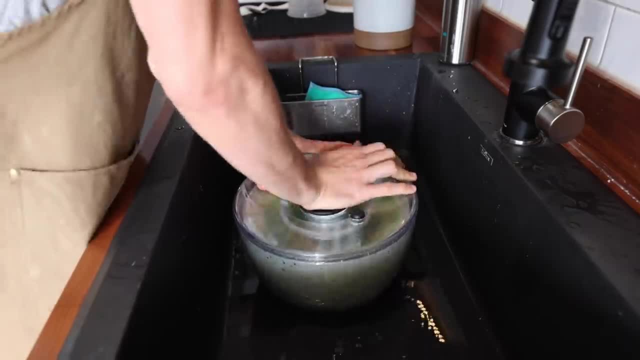 nice heads of lettuce, whatever's looking fresh at the market, and then I get that prepared so I put it through the salad spinner, wash it off, dry it off, put it in a bag so that's ready to be added to the salad. I like to put in some meat, some carrots, so I can just add whatever I. 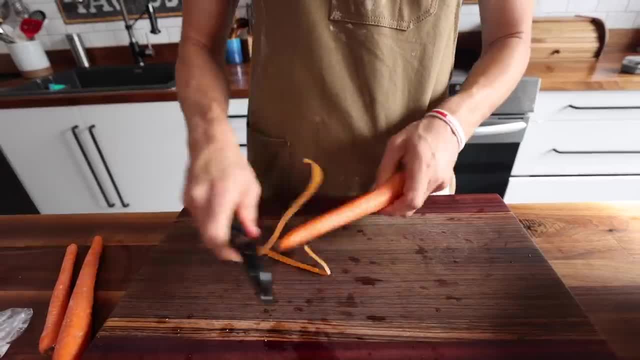 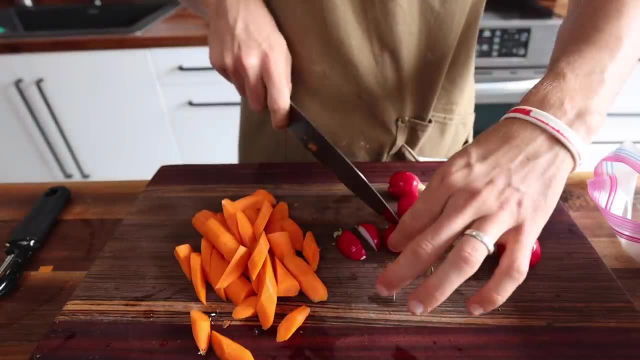 want to the salad, so I can add some carrots and some green onions, some chives and some onions, and I'll add that to my salad and then I'll just switch it over to my oven and I'll just freeze it for a couple of days and then I'll just put it back in there and just let it. 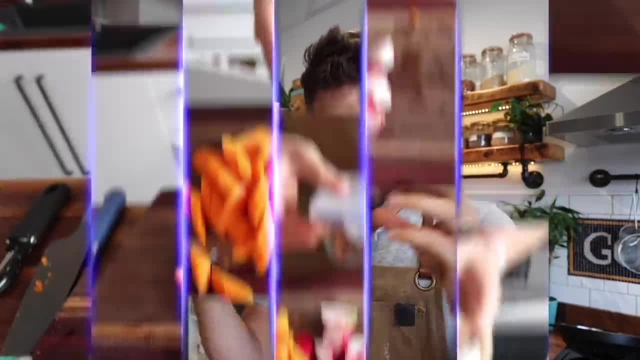 core right in, And then I'll just cut some salads into small pieces and I'll let them harden for a couple of days so I can just keep up with my diet. So I've got a few salads in the fridge. 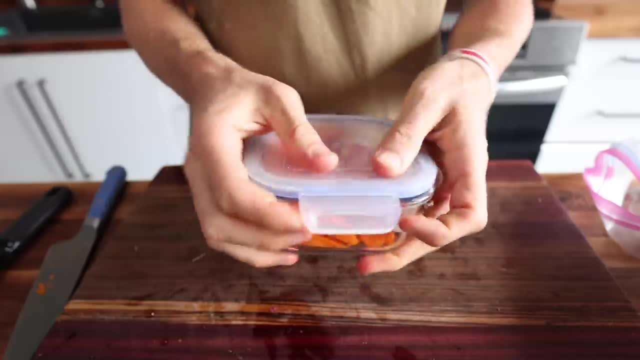 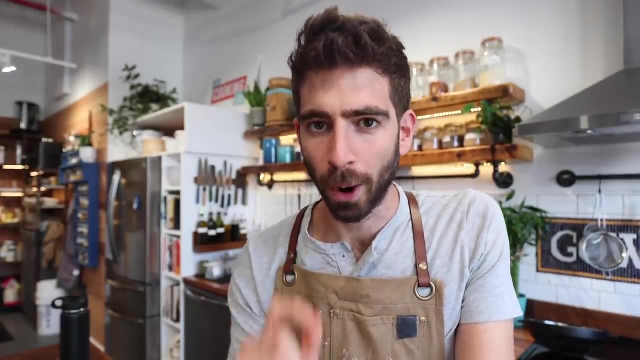 and I'm just going to do that now. I've got the same salad I did two weeks ago and then I'm going to snack on that. you know I'm sick and tired of people saying that in order to bake well, you need to follow recipes perfectly. there's definitely some truth that, if you want, you know perfect. 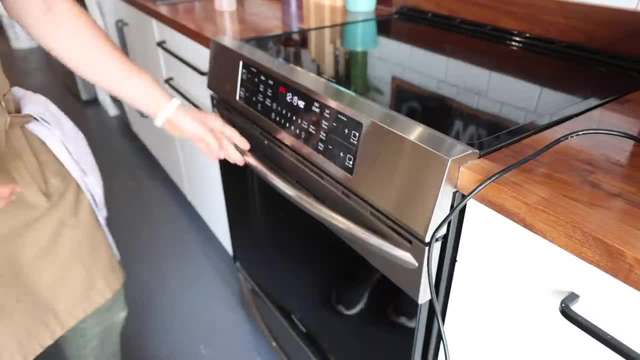 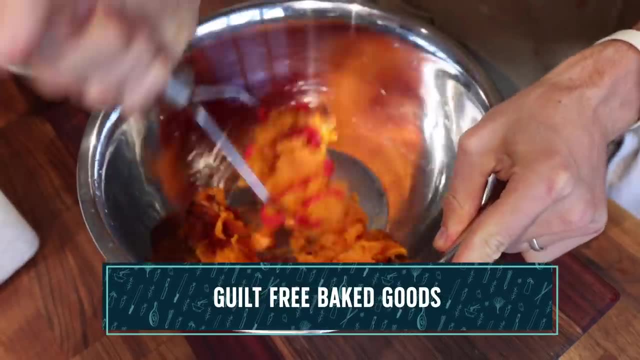 results every time, but for me I bake every single week. I make some type of baked good- a brownie, banana bread, a muffin- and I don't follow any recipes, because I like to use what I have in the pantry and also I like to incorporate more healthy stuff into it where possible. 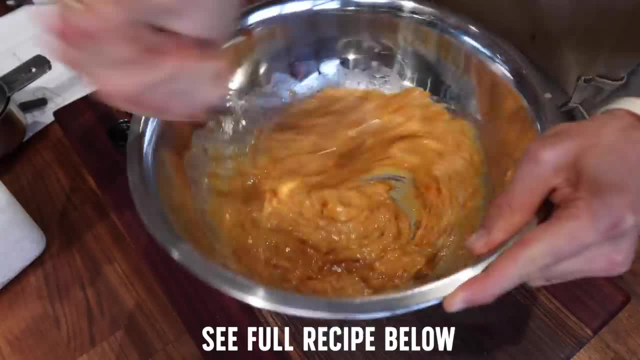 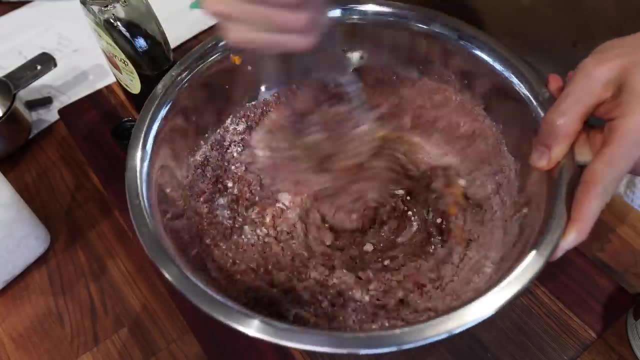 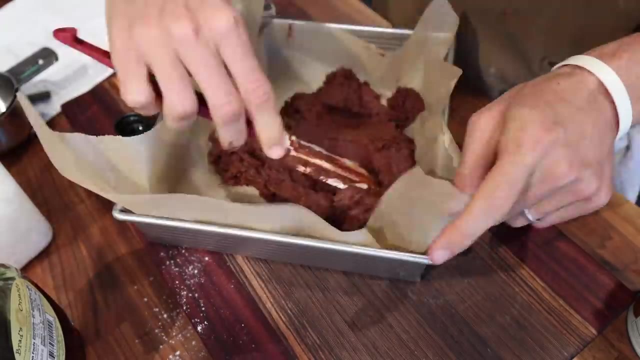 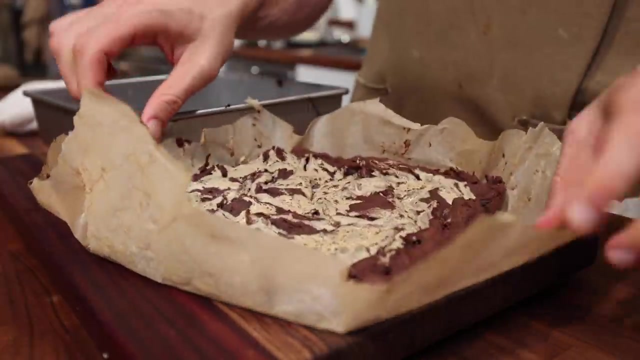 because it is amazing to have a baked good for breakfast or a snack in between dishes. so I do pretty much bake every single week. so here are my sweet potato tahini swirled brownies. one of my biggest pet peeves are people that don't take. 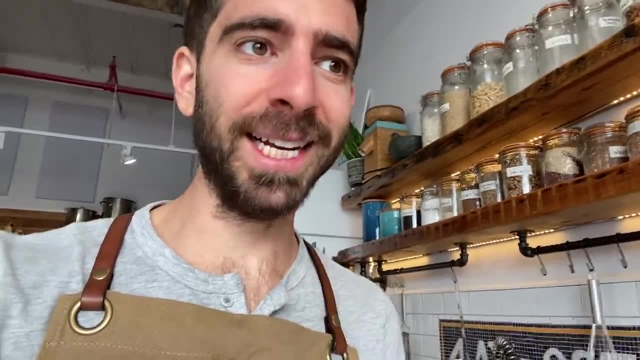 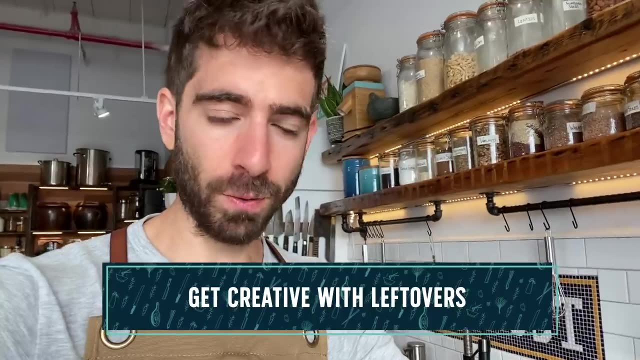 advantage of leftovers. you'll know what the reason for this is, but if you want to make it as a pro home cook, you've got to start getting creative with your leftovers, looking at what you have in the fridge and putting it to use. throw out the recipe and start getting weird with it. 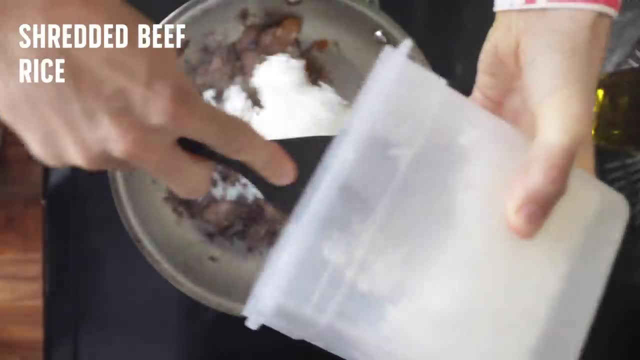 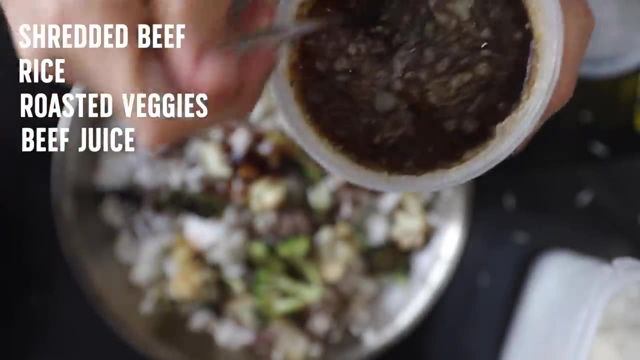 so, after a few days, after you've gone through those main dishes that you prepared, well, check out your inventory and put your brain to work. so, for me, I had some extra meat, I had some extra rice, I had some extra veggies. so what am I going to do? 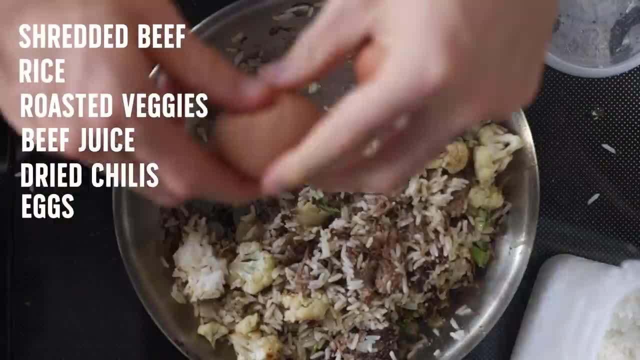 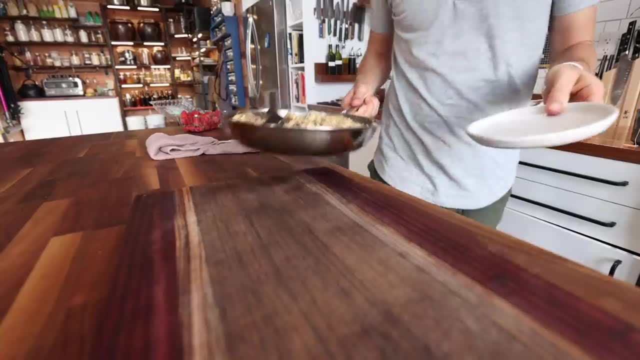 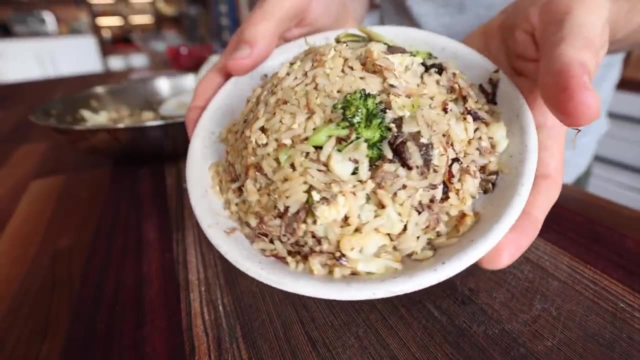 well, the first thing that came to my mind was fried rice, because I did have a few eggs as well. and right there, I just made you know one or two lunches or dinner or whatever you want to use it for. get creative with those leftovers. the last mistake I see when it comes to food prep is 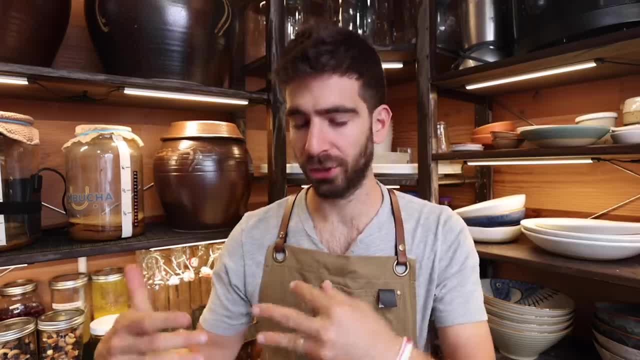 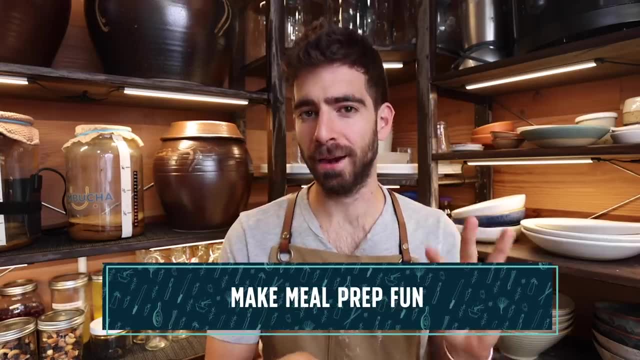 thinking that it's a chore. we've got to get out of that mindset, because if you're stuck in that mindset, well, you're not going to be very motivated to get in the kitchen. so just five quick tips to break out of the chore mindset. number one is make cooking a little more fun. listen to a podcast, throw on some music- there's